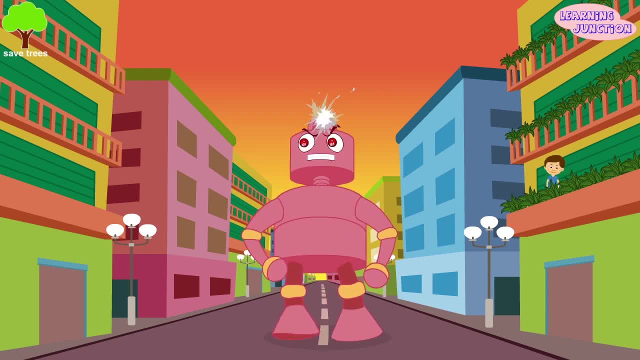 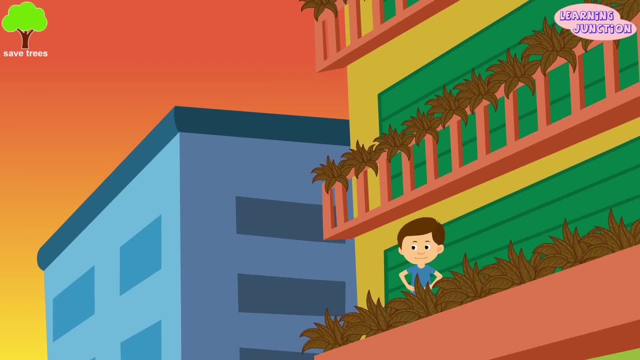 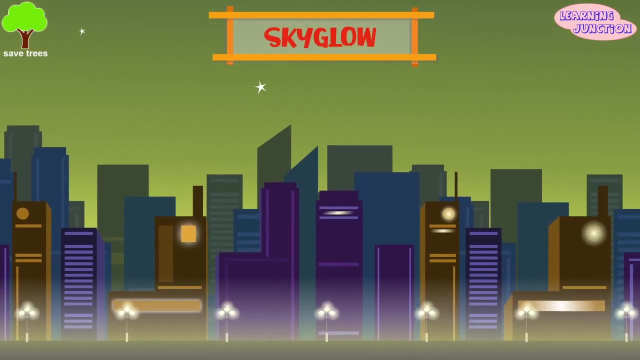 or artificial lights. In simple words, this means too much light. Several species, including plants, animals and humans, are badly affected by light pollution. Um, now let's see the components of light pollution. Sky glow- This is when too many artificial lights cause the night sky to glow. 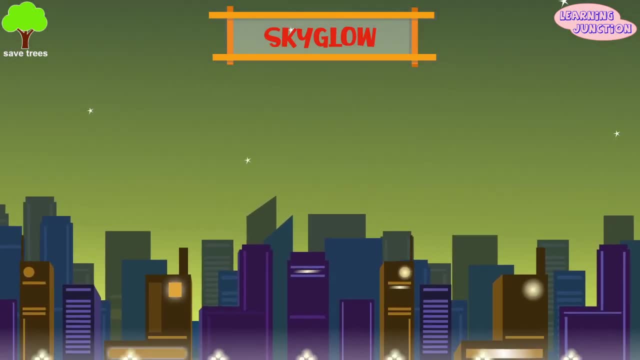 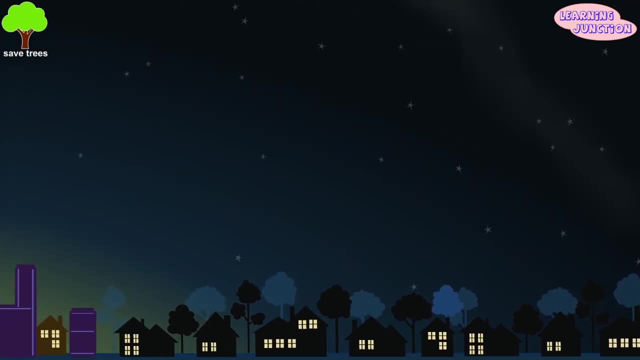 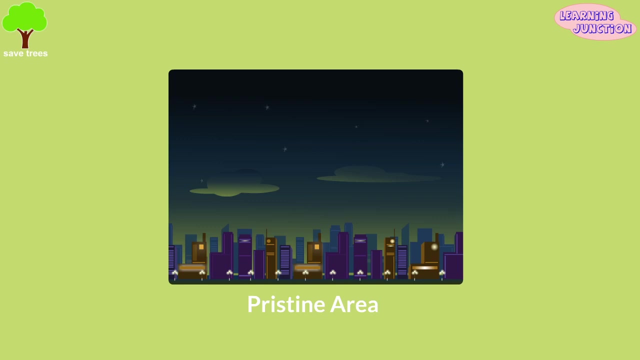 You can easily notice this when looking down at a well-lit city. The sky above the city is too brightened and is harmful for all the species. Light pollution dramatically reduces the visibility of stars. In pristine areas, clouds appear black and blot out the stars. In urban areas, clouds strongly enhance sky glow. 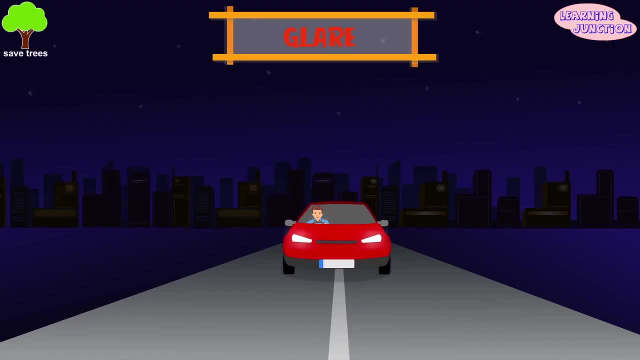 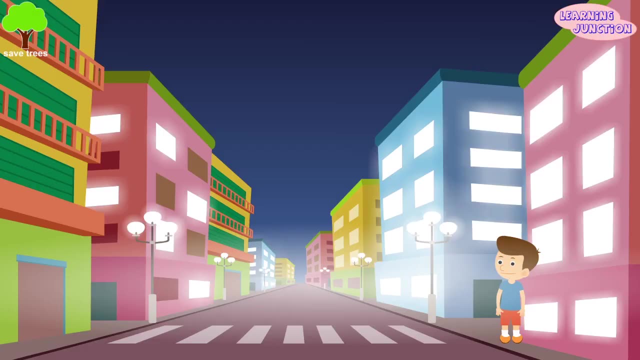 Glare: This is when a light that is very, very bright and often causes glare or visual discomfort when looking towards the light. Oh, no, Clutter. This is when you have too many lights bunched up together or when the lights are grouped in very confusing ways. 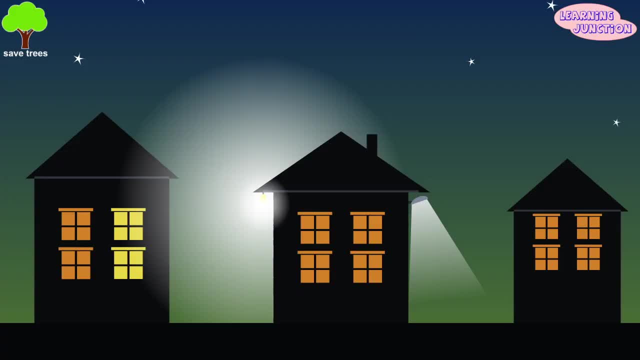 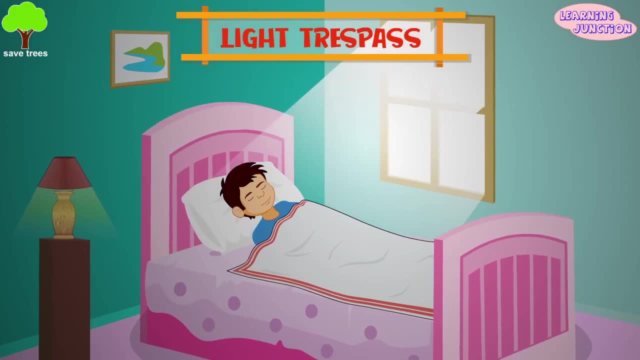 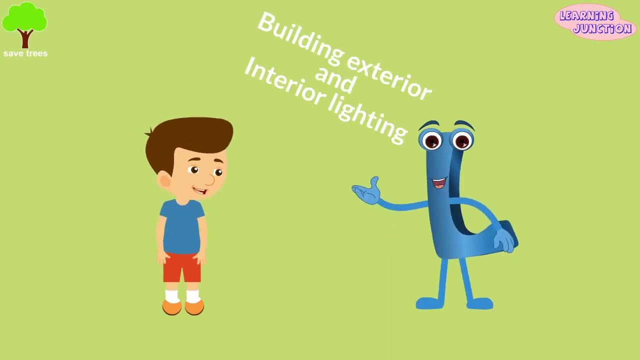 It can make you confused or dizzy looking at them. Light trespass: It is the light falling where it is not intended or needed. How bad you feel when your neighbor's security light is shining through your bedroom windows and lighting up your room all night. Sources of light pollution include building exterior and interior lighting. 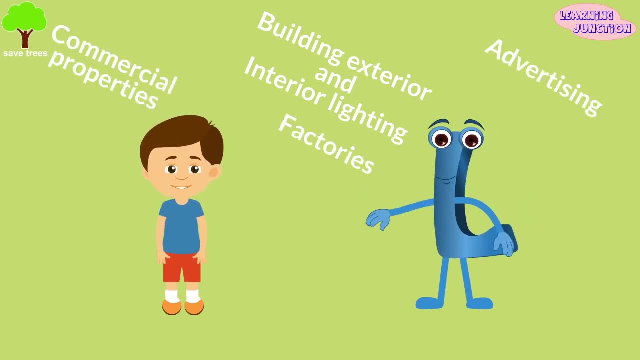 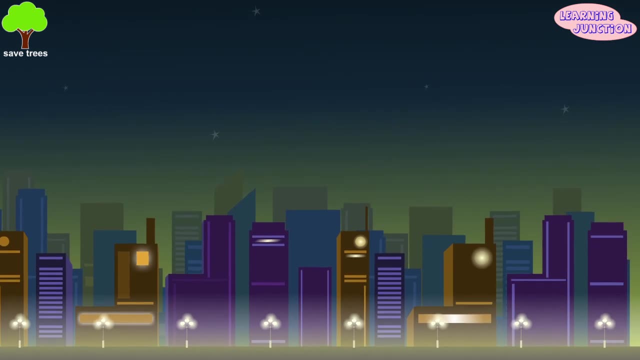 advertising, commercial properties, factories, offices, street lights and illuminated sporting venues. We need light at night, but the fact is that too many light sources are not enough to create light. Too much outdoor lighting used at night is inefficient and completely unnecessary. 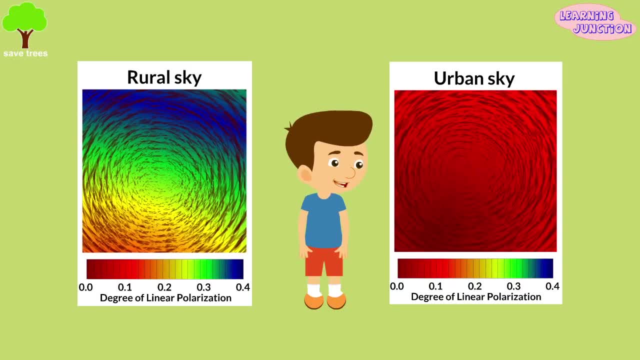 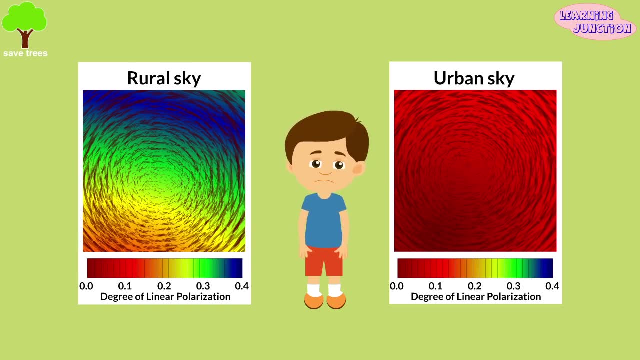 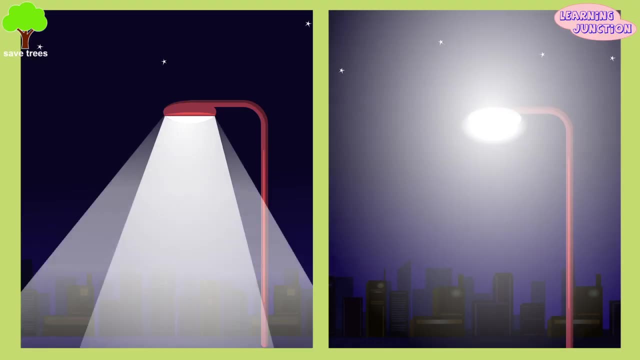 This light and the electricity used to create it is being wasted by spilling it into the sky rather than focusing it onto the actual objects and areas that people want illuminated. This kind of LED drop light could reduce unnecessary light pollution in building interiors. We should ensure that light is only directed below the horizontal. 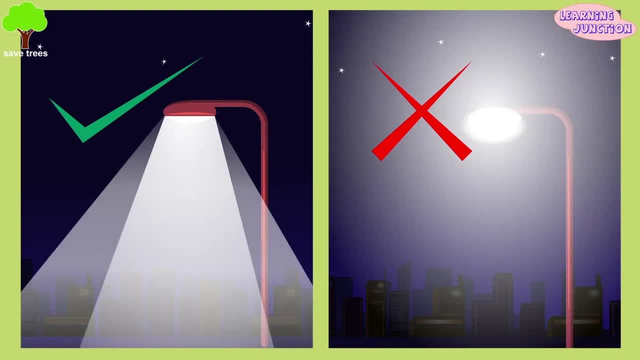 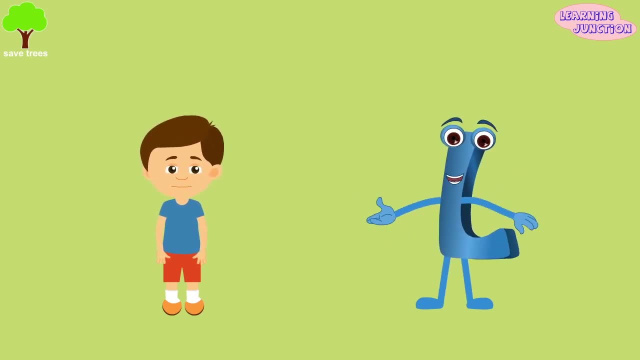 which means less light is wasted through directing it outwards and upwards. Light pollution affects every citizen, increasing energy consumption, disrupting the ecosystem and wildlife, harming human health and also affecting crime and safety. So we should try to reduce this. Bye, bye.